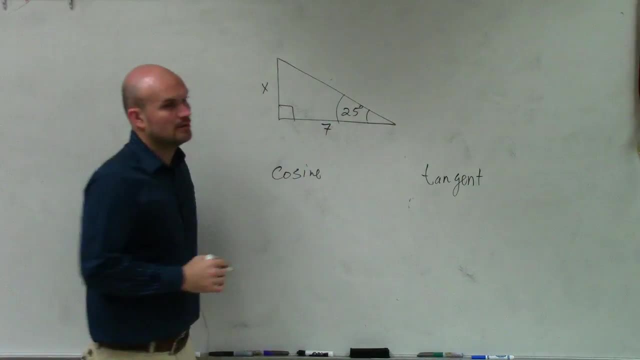 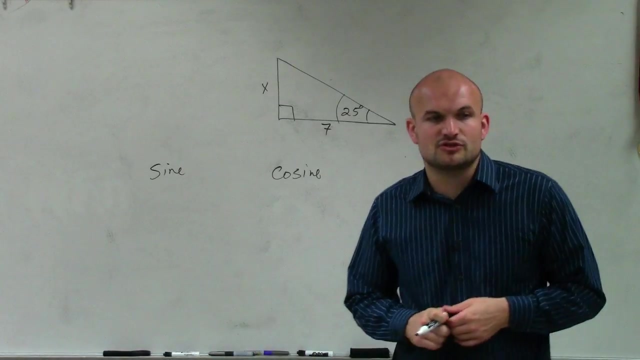 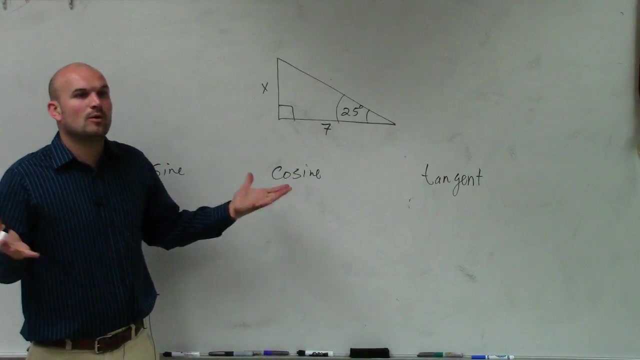 this angle? this is not a number based on this angle, Brandon. what side lengths of the triangle do I have, The adjacent, the opposite or the hypotenuse Based on this problem? what piece of information are we provided? We are provided the adjacent side right, And then 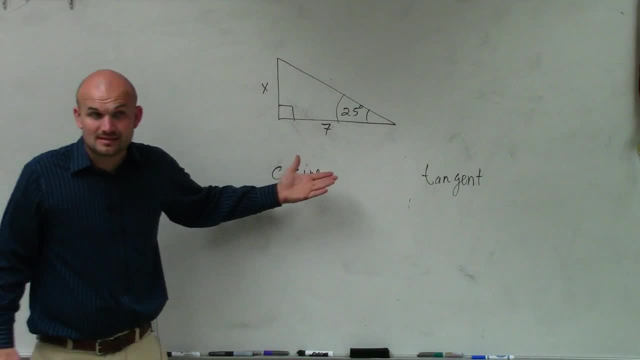 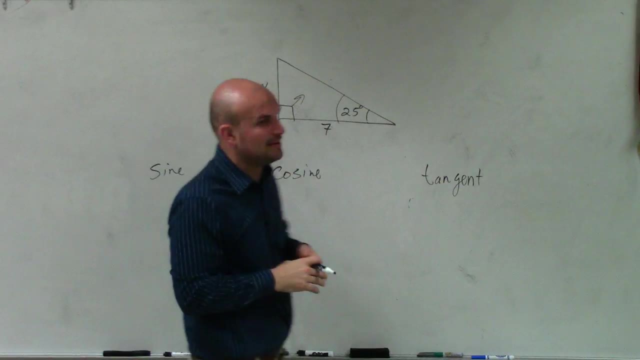 what are we trying to solve for Opposite, The opposite. Hypotenuse is always right across there, right? We don't even. hypotenuse is not even a part of the problem. We're only concerned about the opposite and the adjacent. 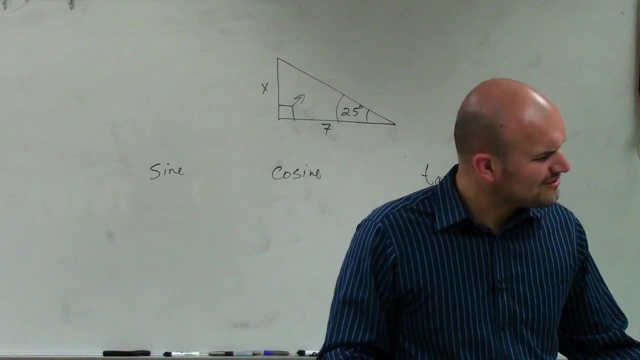 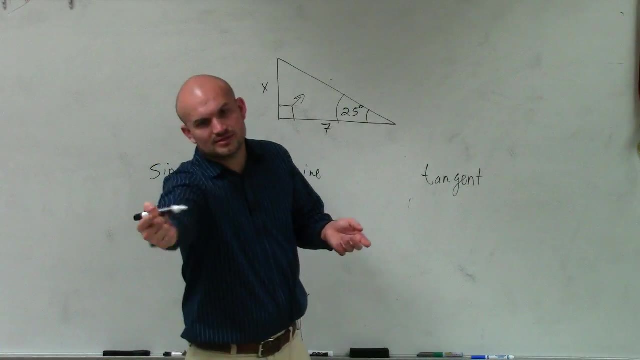 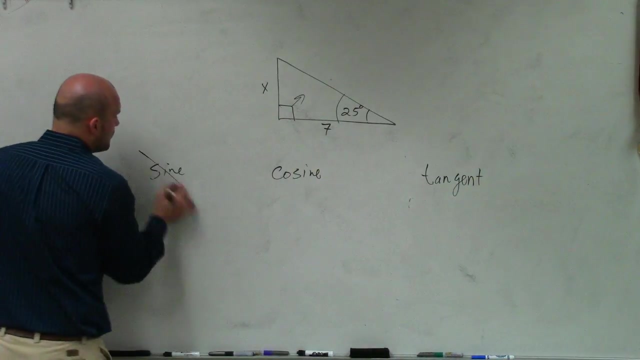 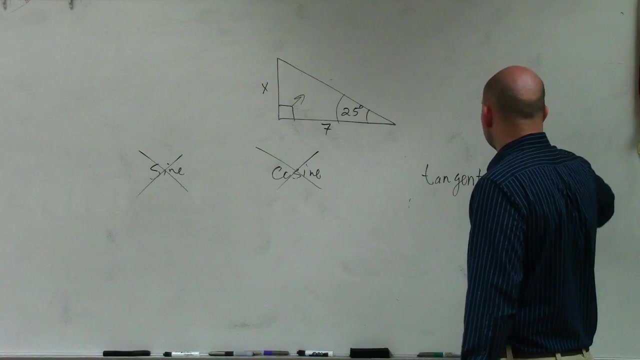 So then I beg the question: Dustin, what trigonometric function only deals with the opposite and the adjacent Tangent function? So we're not going to do sine, We're not going to do cosine, We're just going to do tangent, because tangent 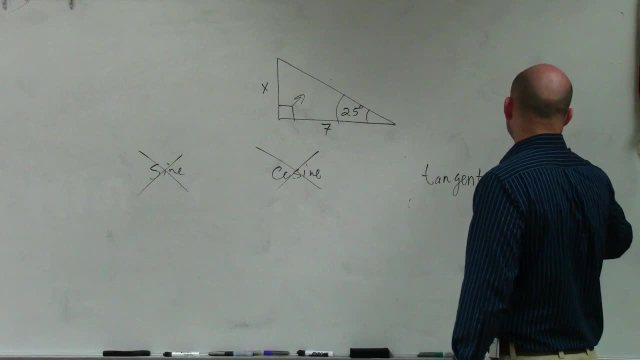 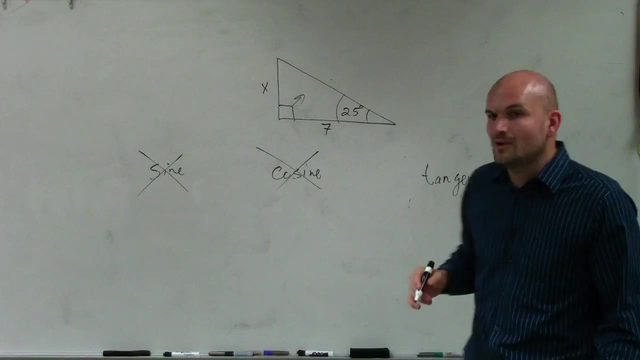 of any angle is equal to the ratio of opposite over adjacent. So in this problem it's nice because you don't have to do one function, But we're actually going to solve. So the way we write this is: it's not any angle, though. 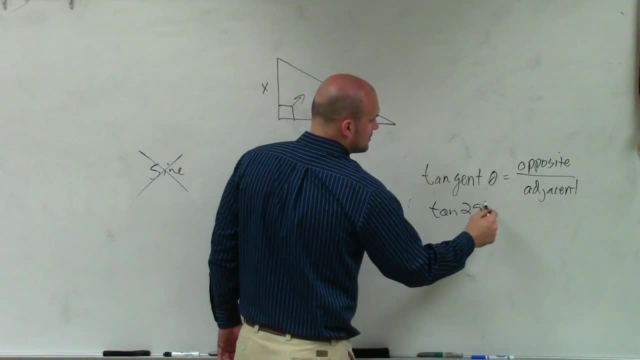 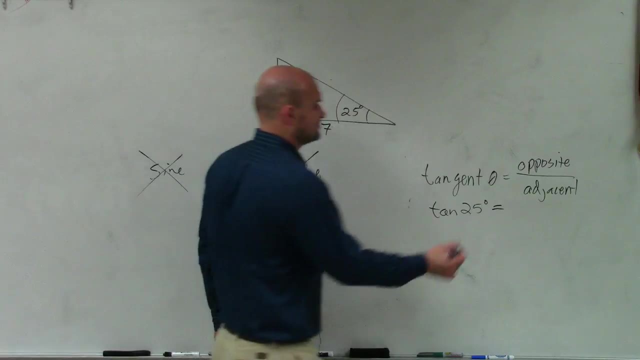 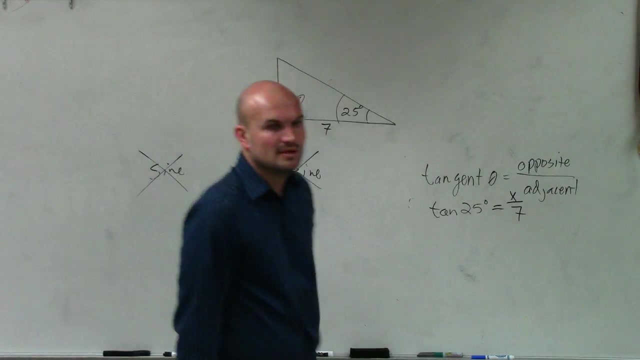 This is the tangent of the angle, 25 degrees, And that's equal to what is the opposite side x What is my adjacent side, 7.. Now, just like any other math problem, tangent of 75 degrees, guys is going to give us a number. 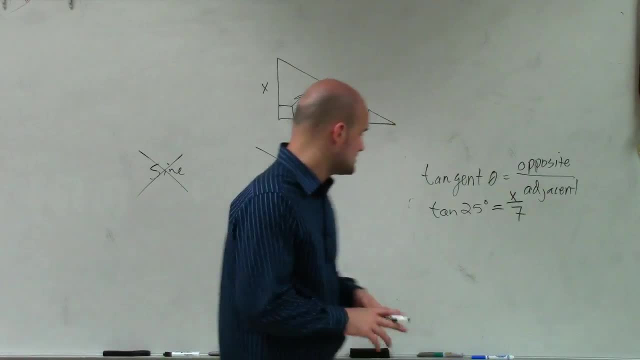 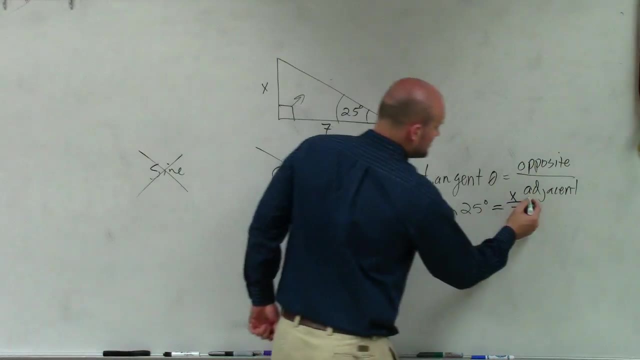 Or tangent of 25 degrees is going to give us a number. So we need to solve for x. So to solve for x, we need to get the x off the bottom. So to do that, I'll multiply by 7 on both sides. 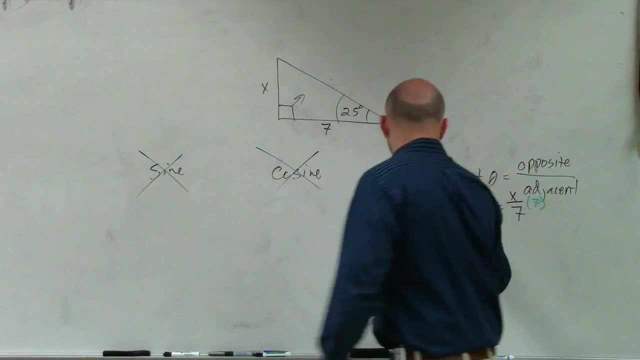 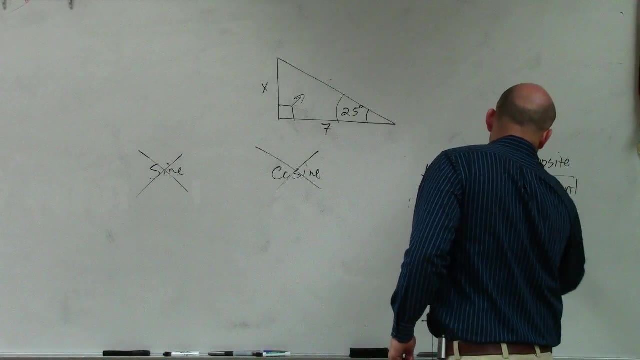 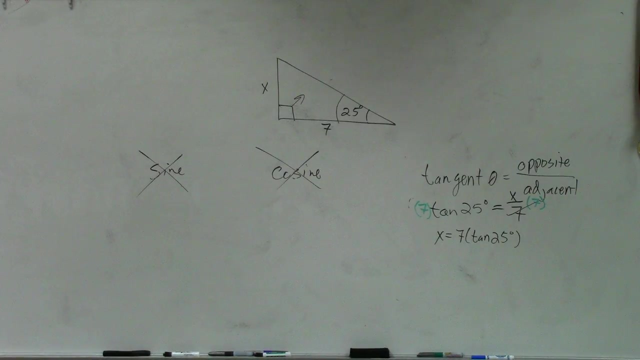 And therefore what I have now is an equation: x equals 7 times the tangent, The tangent of 25 degrees. Now we can figure out the answer for this. ladies and gentlemen, That's not going to be how we're going to leave it. 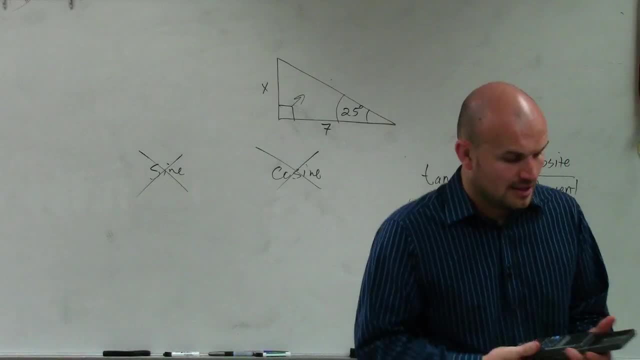 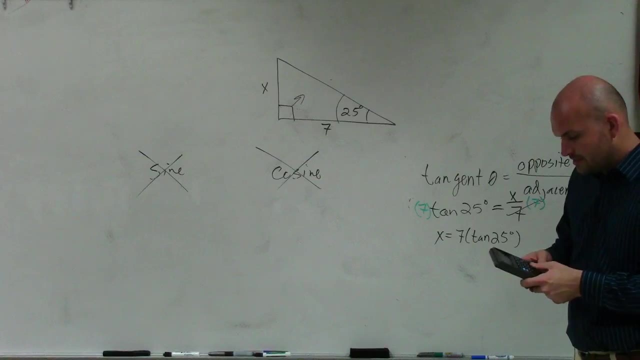 We are going to need at least a scientific calculator to do this, And we're almost there, ladies and gentlemen. So what I'll simply do in my calculator is I'll type tangent, or 7 times the tangent of 25 degrees.